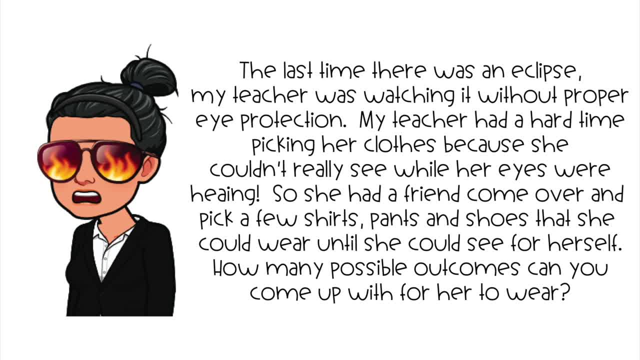 For the next week I had to wear dark sunglasses and I had a hard time seeing until they healed. I had a friend come over and pick out a few clothing items that I could mix and match for the rest of the week at school. My friend ended up picking out two tops, a t-shirt and 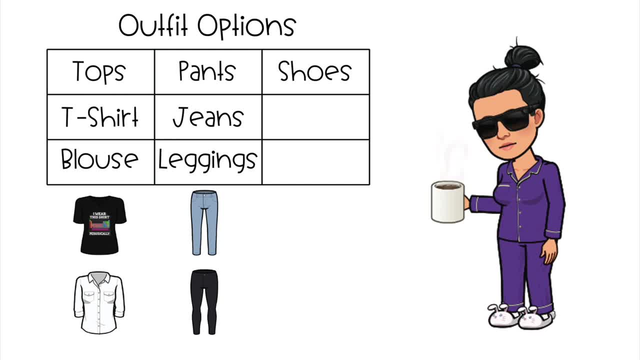 a blouse, two pairs of pants, jeans and leggings, and two pairs of shoes, runners and a pair of flip-flops. Let's use this situation to figure out the possible outcomes. In other words, how many possible outfits can I get with the items that she selected? 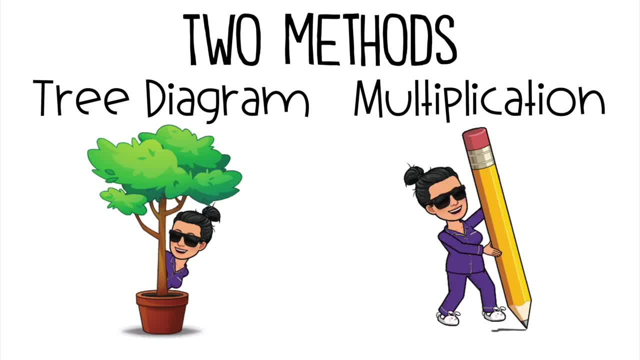 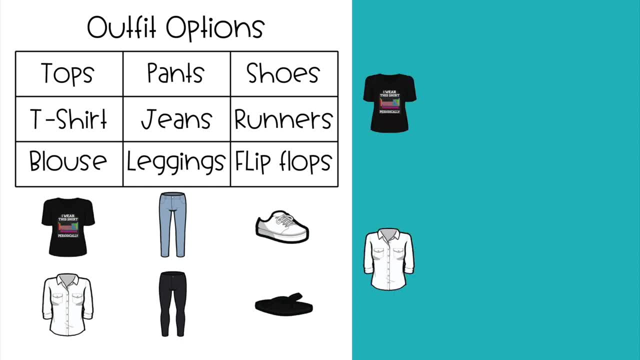 We can do this in two ways: With a tree diagram or by multitasking the options. let's start with the tree diagram first. let's start with our shirt options: the t-shirt and the blouse. now let's add some pants. we have our jeans and our leggings. last we have our shoes, a pair of runners and our flip-flops. now 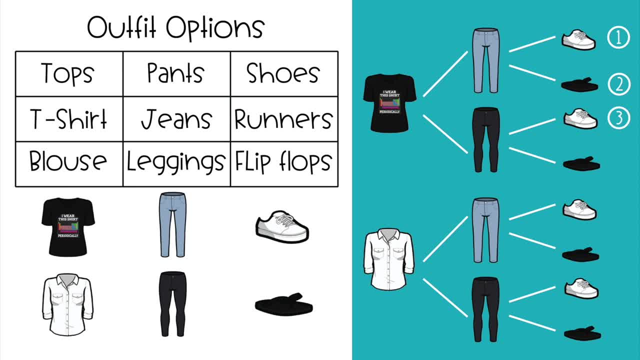 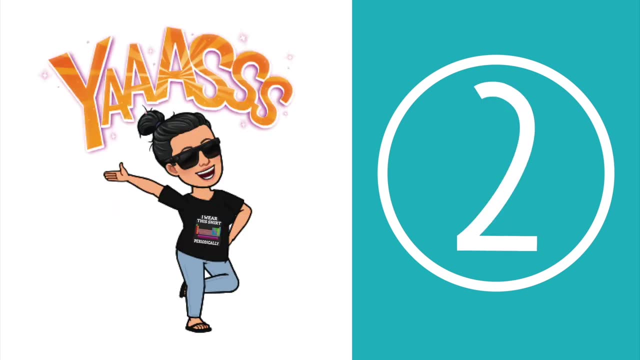 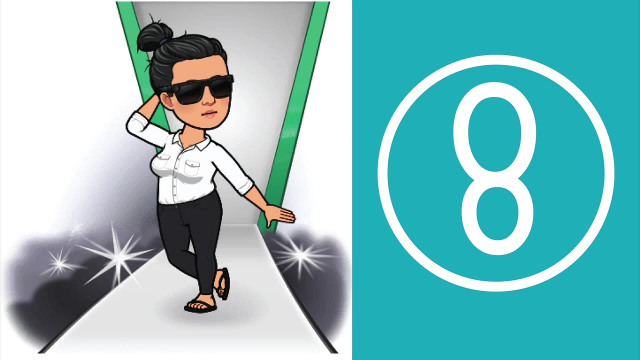 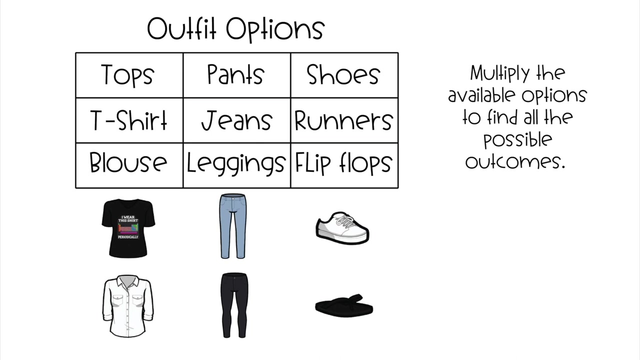 let's count them up: one, two, three, four, five, six, seven, eight. that gives us a total of eight possible outcomes. let's check to make sure. here's our first combination, second, third, fourth, fifth, sixth, seventh, and that makes eight. let's look at how we can use multiplication to solve this problem too. again, let's start. 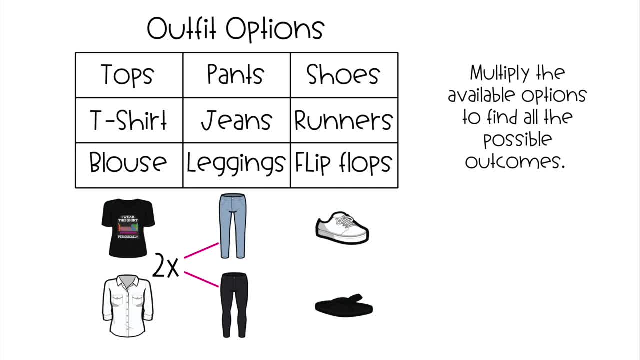 with our two tops, then we'll multiply by our two pairs of pants and we get four from there. we're going to add a pair of pants and we're going to add a pair of shoes. that makes eight and that gives us a total of eight possible outcomes. 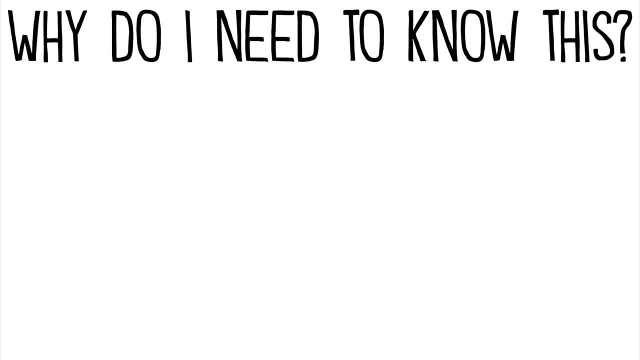 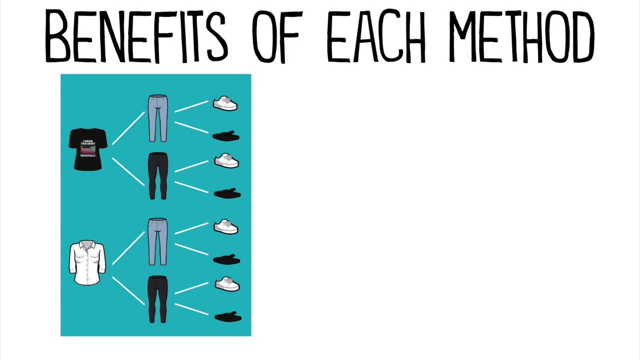 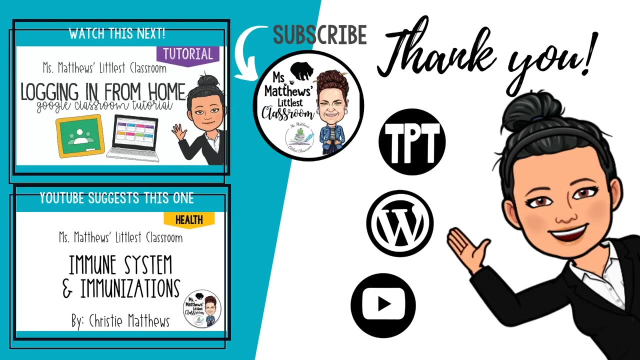 these kinds of problems will inevitably pop up in your lifetime, like when your insurance premiums are calculated, and even in games of chance. you can do the calculations with the tree diagram if you prefer to have a visual, but the multiplication method is the fastest option. thanks for watching. remember to. 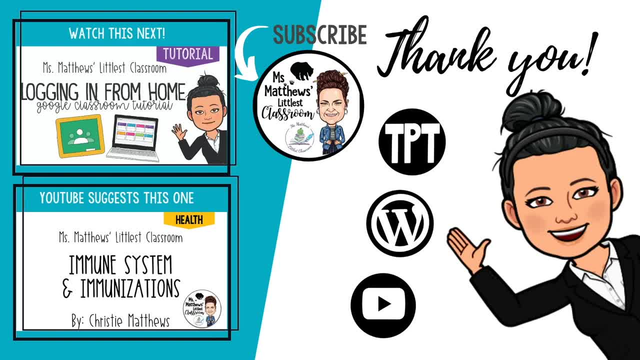 like and subscribe so you'll be notified when I upload my next video. you make good choices.